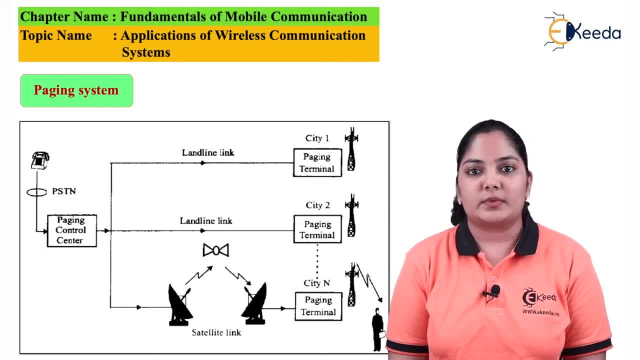 This region depends on the types of paging systems. The area may vary from 2 kilometers to 5 kilometers. The paging systems may carry numeric messages, alphanumeric messages or voice messages. The paging control center forwards the message to the various paging terminals. The paging systems are designed to provide reliable communications to the user, Whether 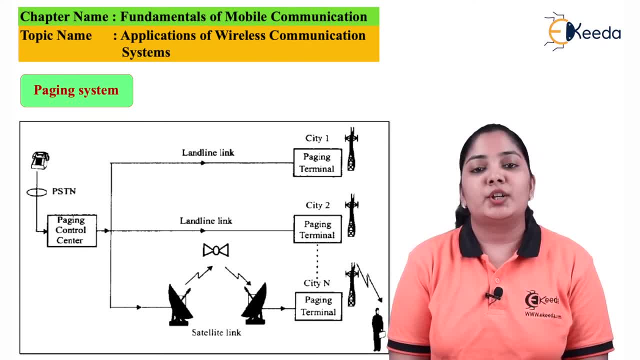 the user is inside a building or under a bridge, it should be ensured that the communication is made Here. high power transmitters are used. The data rate for paging systems is very less, since only few bits of messages are being sent. The next topic that we're going to see. 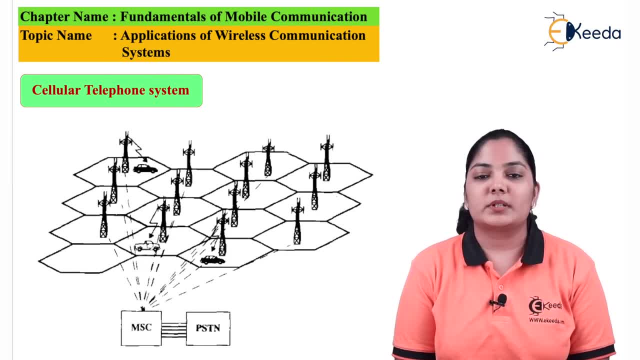 in applications of wireless communication systems is cellular telephone systems. As we can see in the diagram, there are hexagonal cells. These hexagonal cells are nothing but geographical locations in which the mobile will be moving from one place to another. At the center of 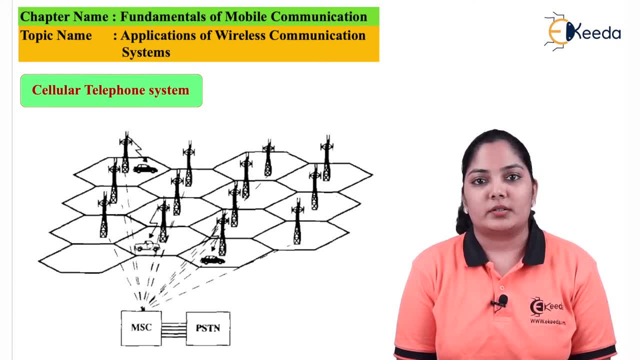 these hexagonal cells we have base stations. These are towers that has transmitters and receivers for communicating with the mobile stations. All the base stations are wirelessly connected to MACs. MAC stands for Mobile Switching Center, also known as MTSO, Mobile Telephone Switching. 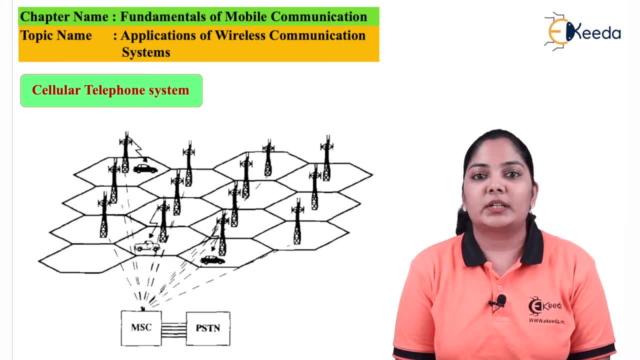 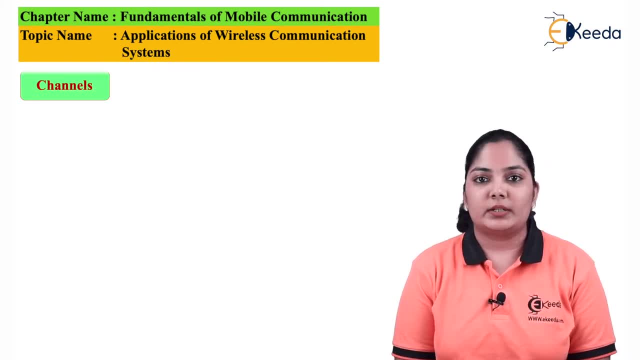 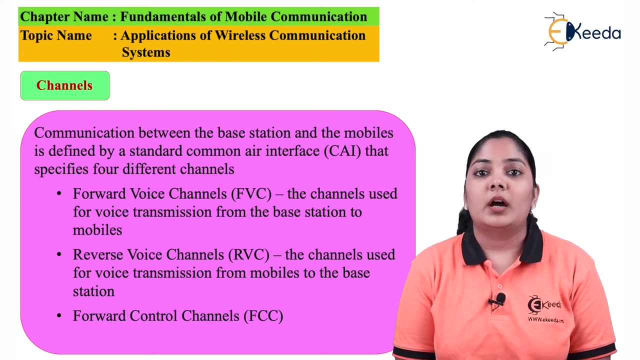 Office. The MAC is then further connected to the PSTN, called as Public Switched Telephone Networks. Each mobile station has a trans receiver, that is, a transmitter and a receiver, to communicate with the base station. A mobile may travel from one cell. 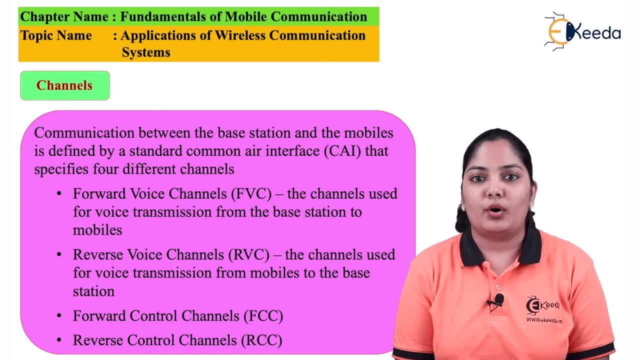 to another cell and during that it may be handed off from a base station of one cell to another cell. Here handoff takes place. The base stations are then connected to the MACs. MAC handles multiple base stations together. At any given point of time, every MAC has.